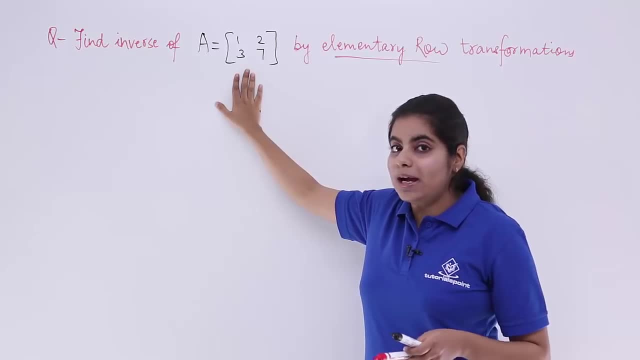 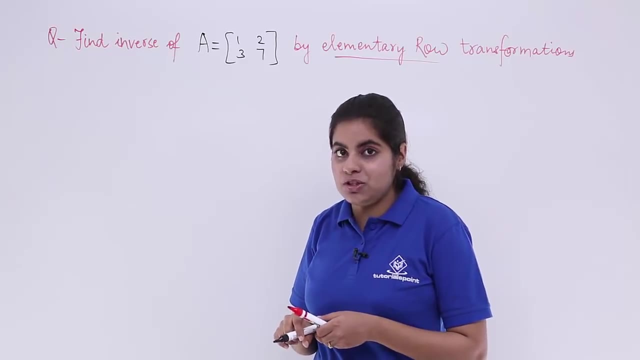 is such that we are being given a matrix A, which is a 2 by 2 matrix, and we are supposed to find out the inverse of that matrix using the elementary transformations. Let's write the heading as solution, and then we will be getting started with our basic problem. I 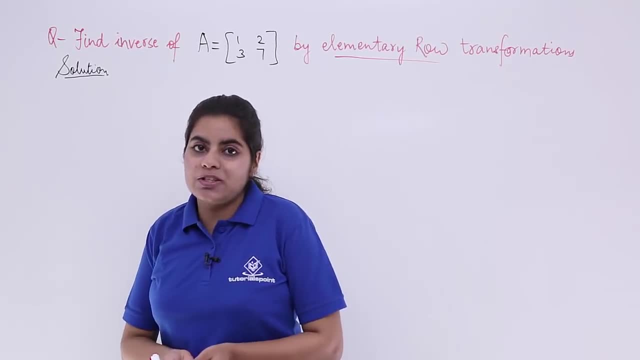 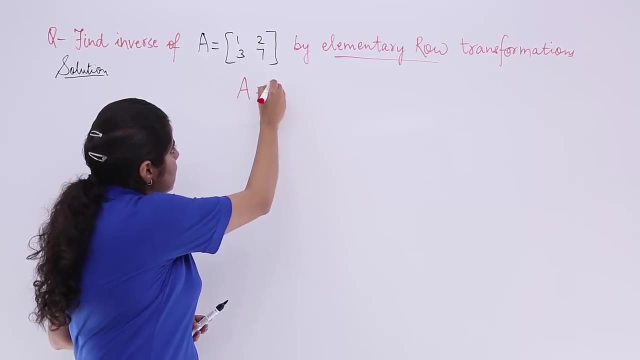 have the matrix and you need to know, in these questions related to elementary transformations, you will be using the formula that the given matrix A is equal to IA. You need to remember this, that we are using this only in case of elementary transformations. So let's see. 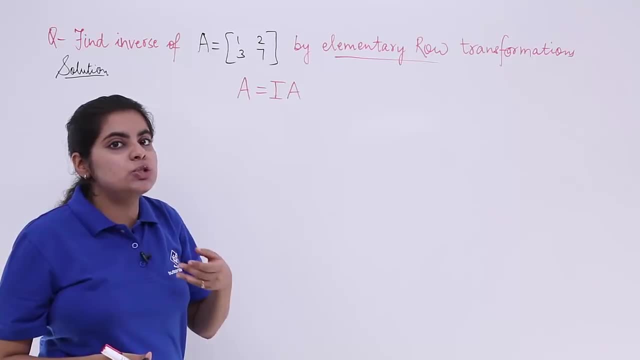 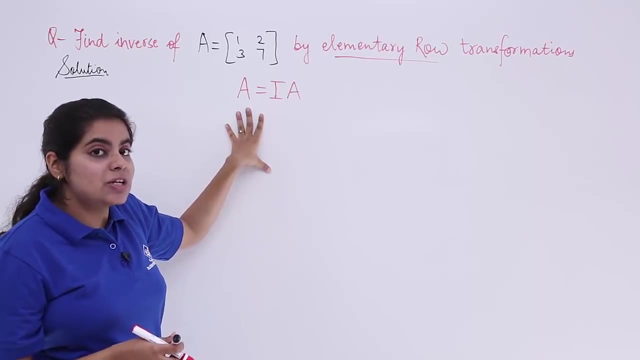 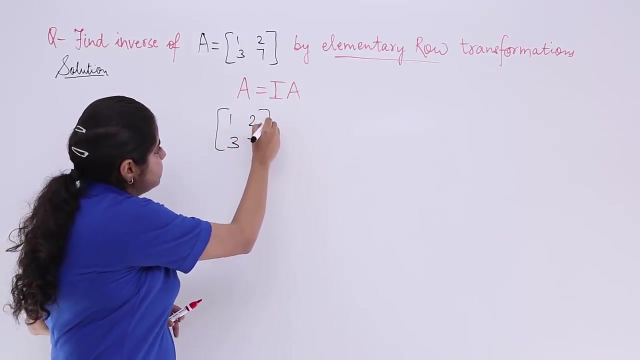 the case of row transformations In column transformation, the situation will get different. It will become: A is equal to AI. Now, what was the I matrix? I is identity. What is the A matrix? A is 1,, 2,, 3, 7.. So it is 1, 2,, 3, 7.. What is I? I is 1, 0, 0, 1.. It is 1,. 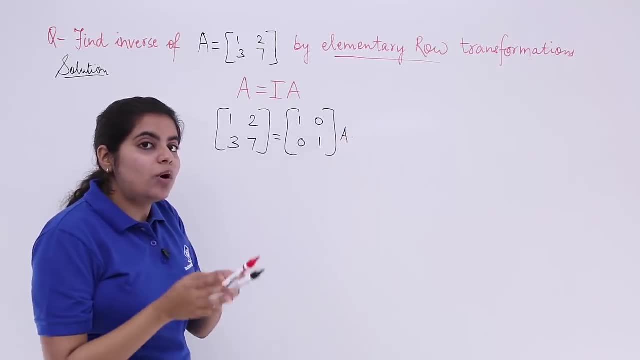 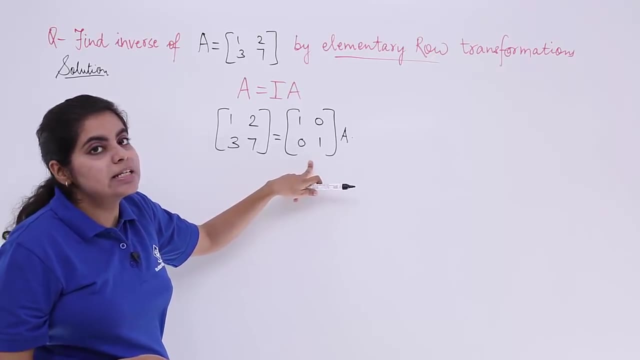 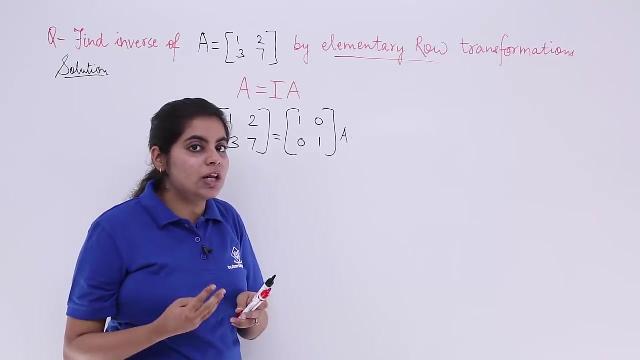 0, 0, 1 and A remains as it is. Now. what is my task? My task is to convert the elements of this given matrix A into the identity matrix using the elementary row transformations. We know there are three transformations. You can interchange the rows and columns. Let's 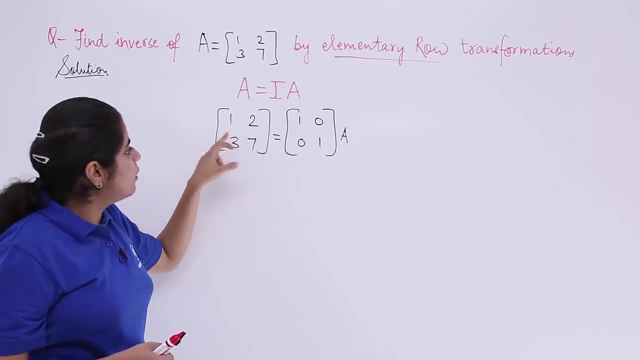 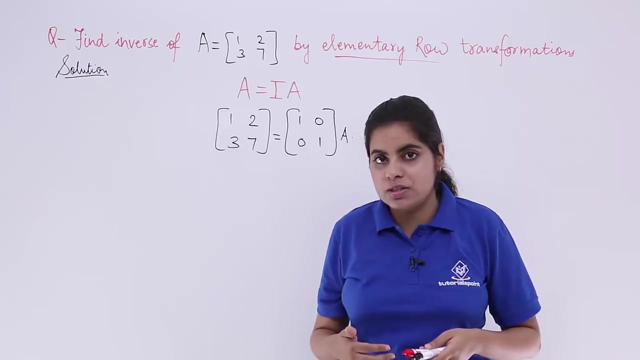 see whether this transformation number 1 fits in the case. If I interchange row 1 with row 2, there is no use because I need 1 here. only 1 is already here. Why to change Column transformations? we cannot apply. So what we are left with, We are left with other transformations, If I apply. 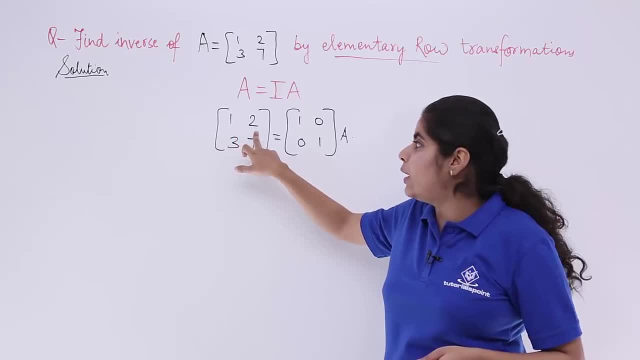 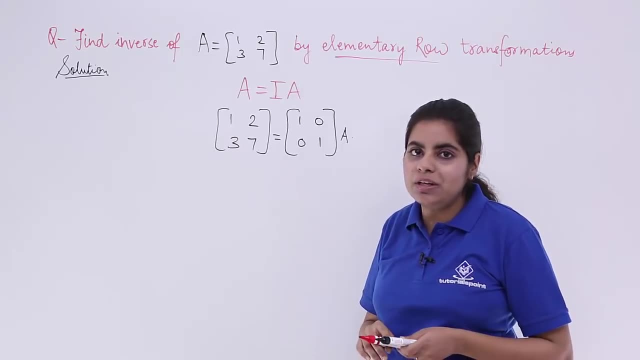 row 1 divided by 2.. So it becomes 1 by 2 and it becomes 1.. Not of any use to us If I apply any other thing. that means multiplication by scalar Again not of any use to us, So let's use our. 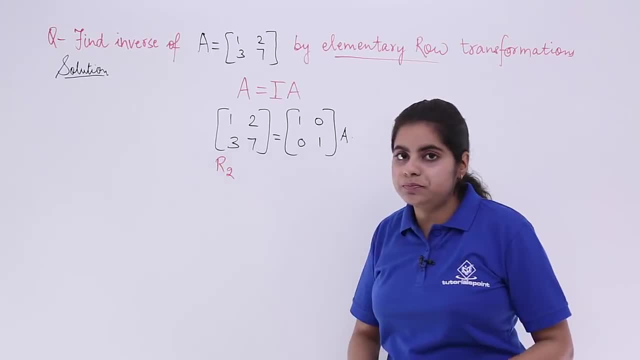 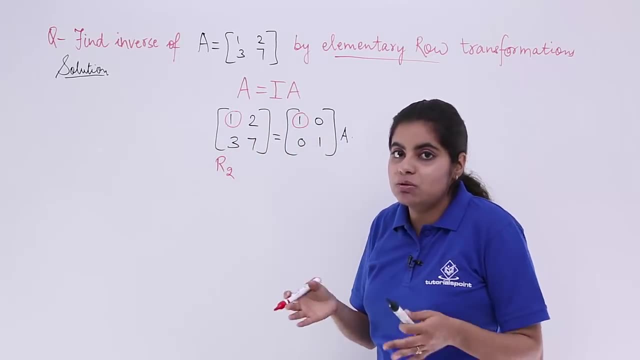 mind and apply something on the row 2.. Why row 2?? Because the first element should be 1. It is already 1. You cannot change it. There is no need to change it. even So, row 2, I apply the. 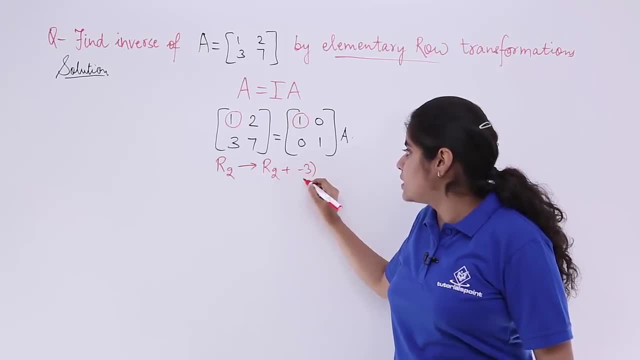 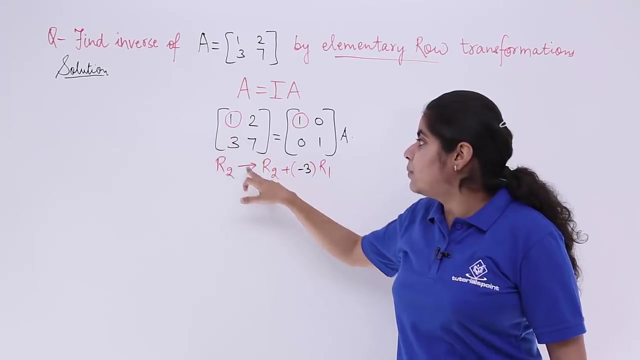 transformation as row 2 plus 1.. Minus 3 into r1.. Why are we using this? Because I know that if I multiply, the situation will change, and minus 3 into r1 means minus 3.. Now, minus 3 plus r2 means minus 3 plus 3, which is 0.. 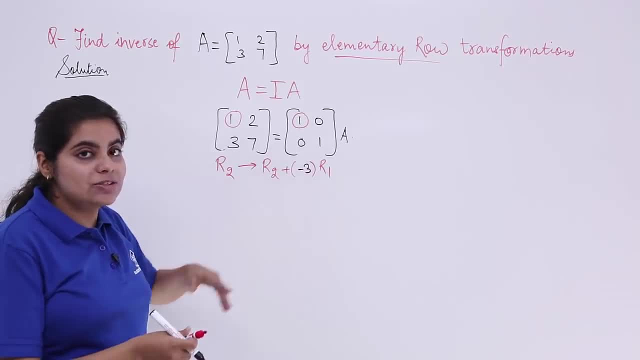 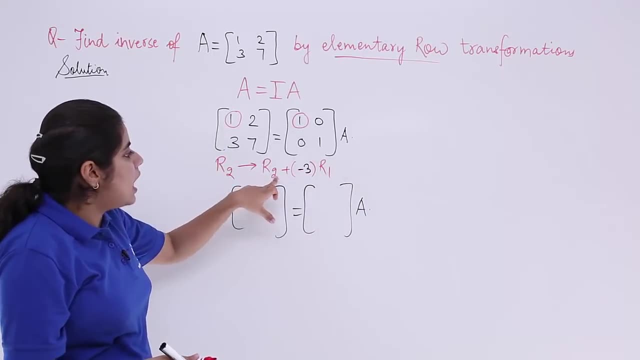 So I am explaining it again. What we are doing is we are applying this transformation and I have some changes which are visible to me, in the manner it is multiplied by A and r2 plus minus 3 into r1, which means minus 3, into the first matrix element. minus 3 plus 3 is 0.. Changes are. 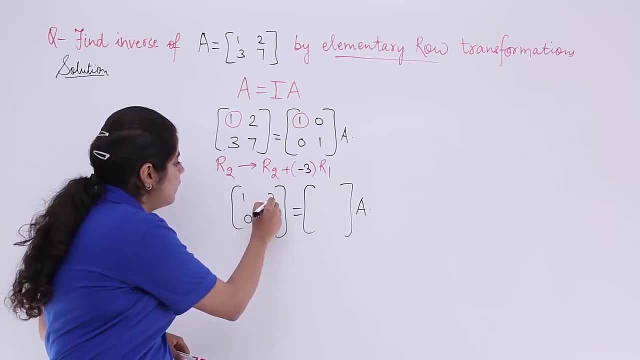 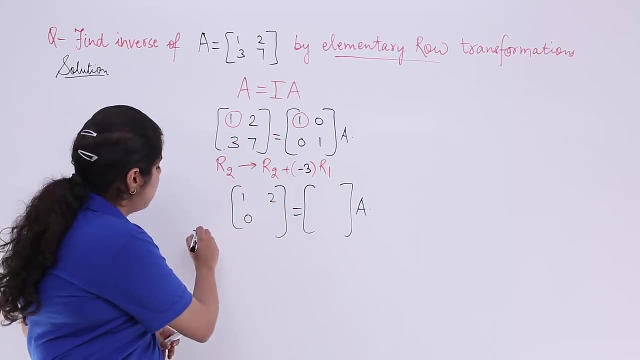 only in r2.. Do not change r1.. Just write r1 as it is. What about 7?? 7 plus minus 3 into 2.. So 7 plus minus 3 into 2.. What happens? It becomes 7 minus 6, which is 1.. So changes are 1 here. What? 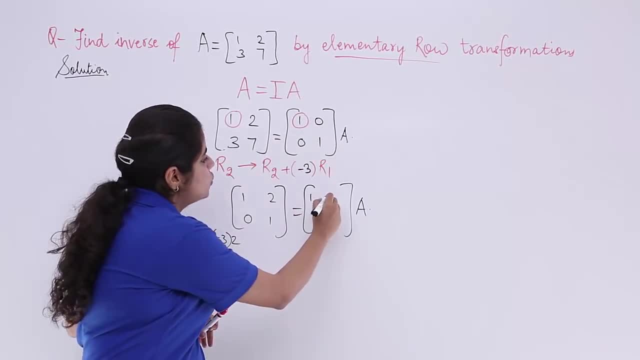 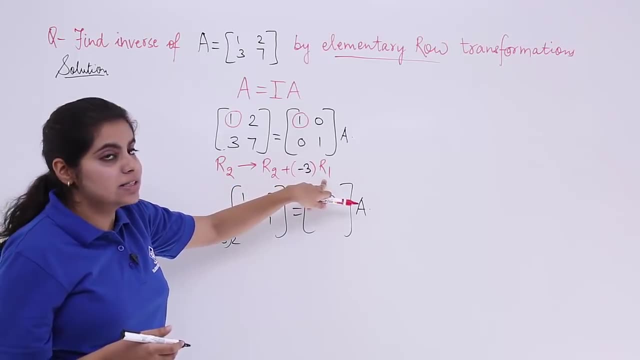 about The second matrix, identity matrix, row 1 does not change, It is 1, 0.. What about the second line, that is second row? It is r2 plus minus 3 into r1.. So 0 minus 3 is minus 3.. Next, here we have 1.. 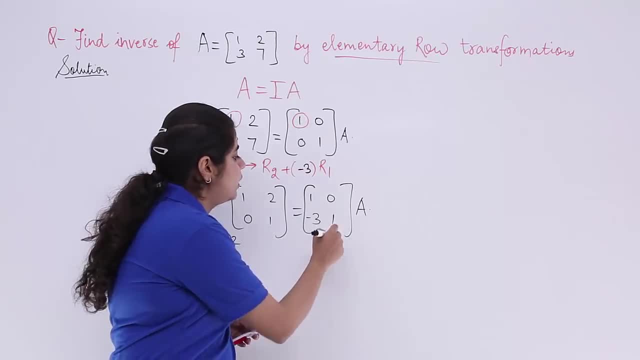 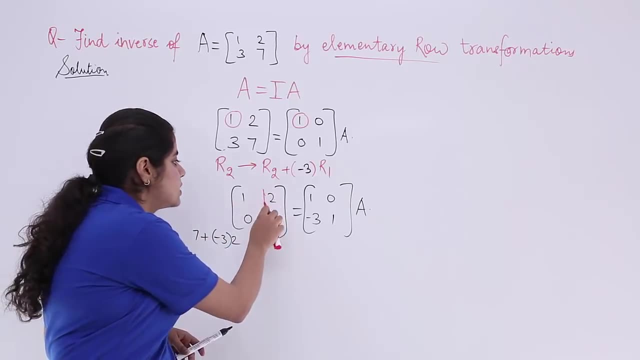 Now 1 minus 3 into 0, which means 1 only. My task is to write it in the form as 1, 0,, 0, 1.. This should be made 0.. This is creating a problem, So we need another. 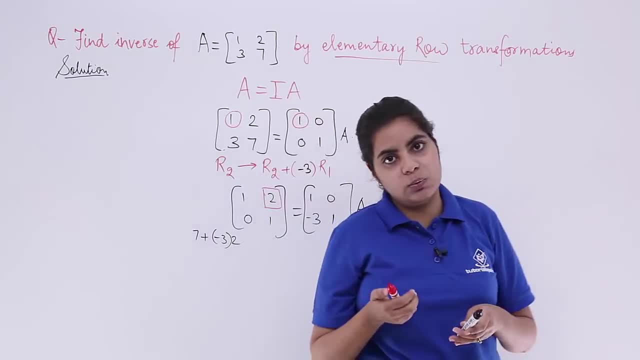 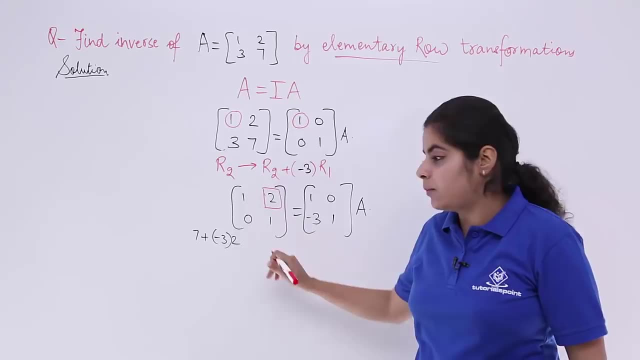 transformation for changing of 2 to 0.. What next operation can be applied? We can apply something on the row 1 now, such that row 1, row 1 changes to row 1 plus minus 2 into r2.. Why are we? 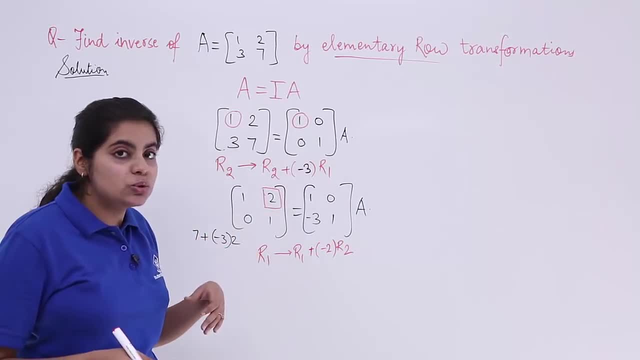 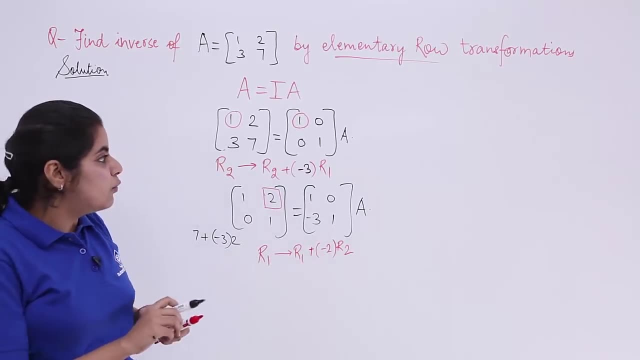 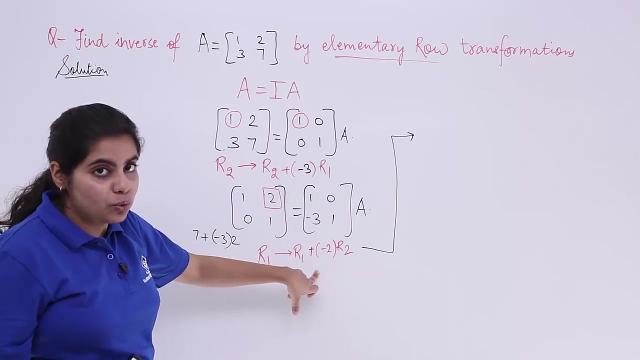 doing this? We are doing this to convert the 2 into 0.. 2 into 0 will be converting only when some operation of this will be applying. Let's see what happens by application of this row transformation. I have operation in row 1..